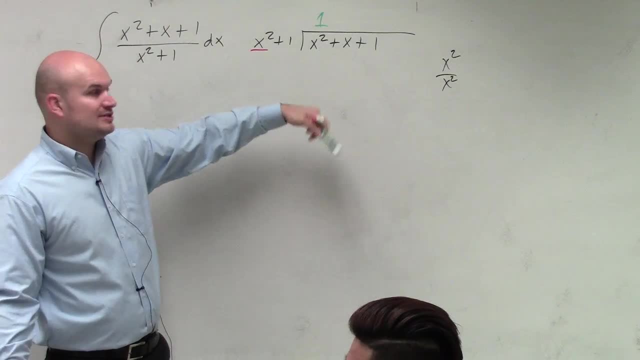 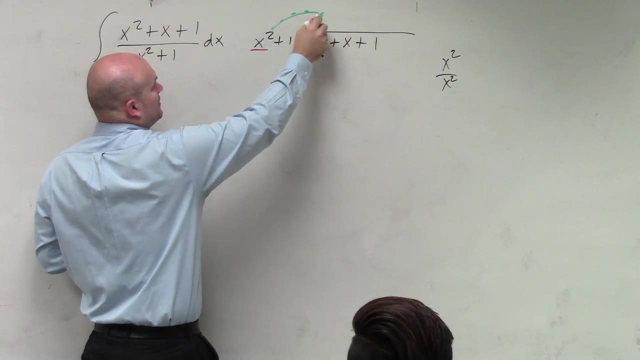 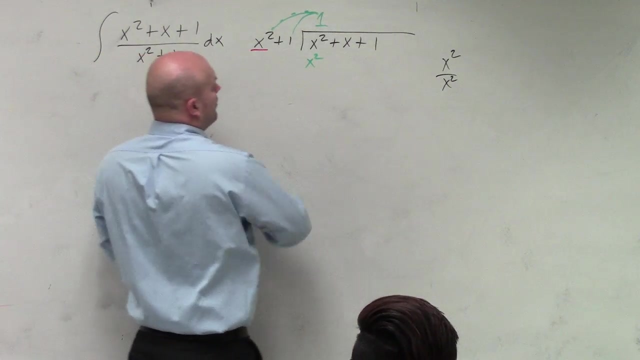 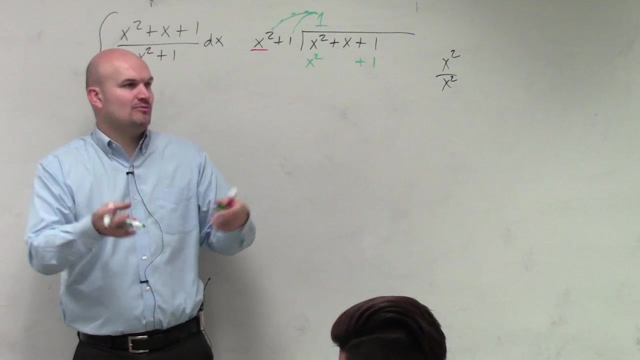 And we can just put that right above there. But then what we need to do is we need to multiply that back over So one. so you've got to multiply this one times the x squared and the one. So one times x squared is x squared. One times one is one. Now I'm going to put that under the common terms because if you guys remember adding and subtracting polynomials, we'd vertically align them because those are like terms. I can't add or subtract one from x. 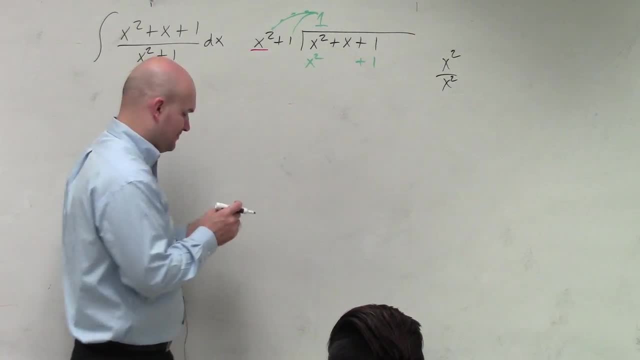 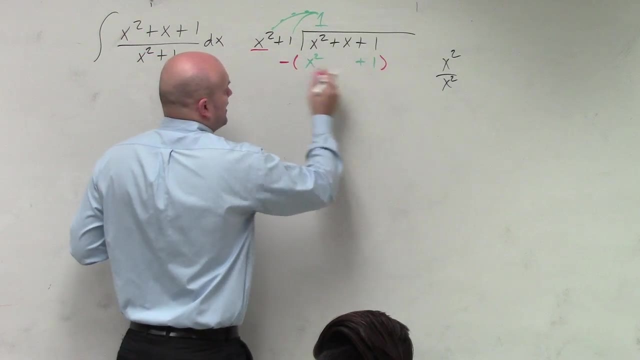 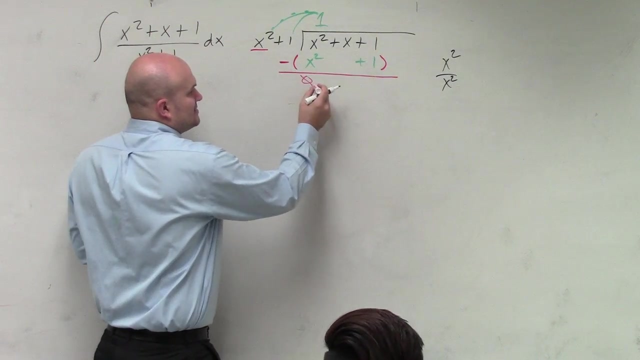 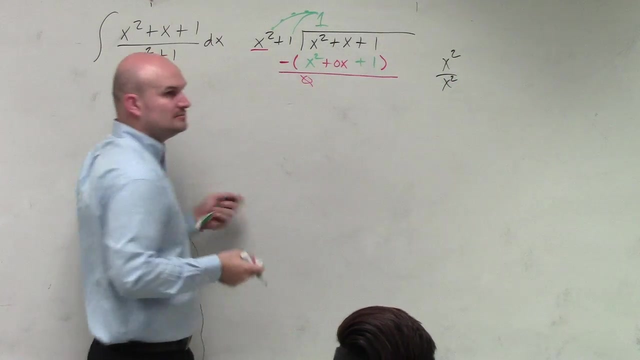 So I can only add and subtract one from one. So that's why I'm vertically aligning them. Then I'm subtracting each one of these. So the way that I like to do it is just say subtraction and then just put them in parentheses. You don't really need to. I mean, you could just say x squared minus x squared, we know, is obviously zero. You could put a filler here and say this is going to be zero x. right, because zero times x is zero. But what is x minus zero x? That's just going to be zero. 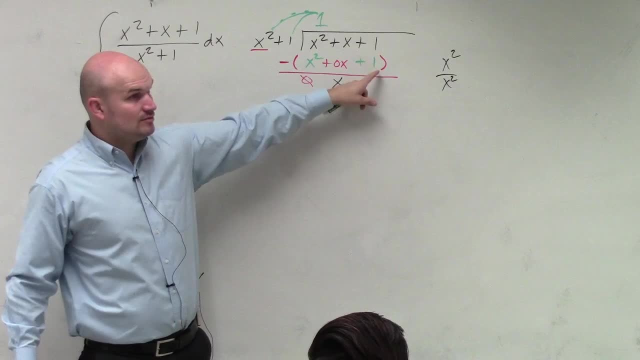 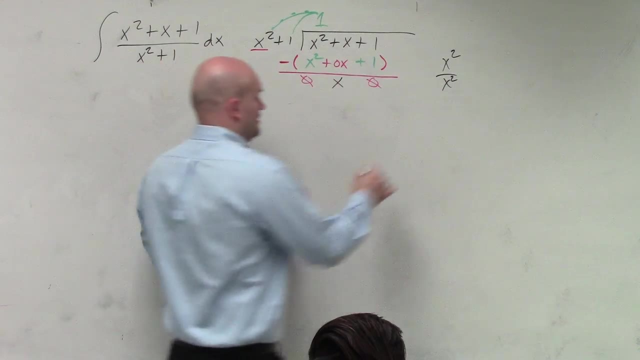 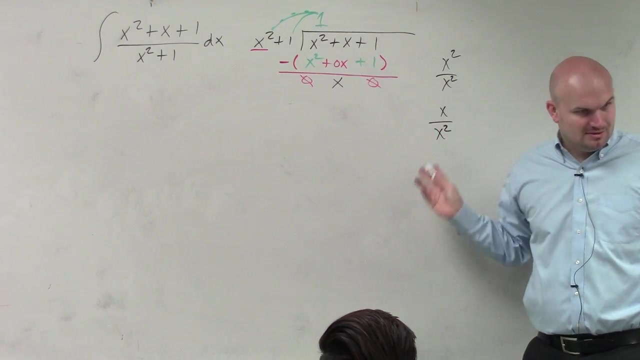 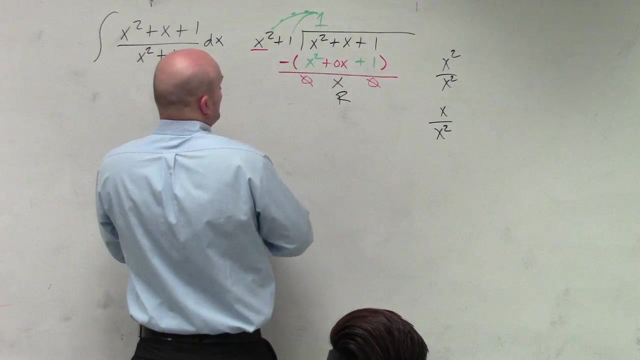 And then one minus one is obviously zero. Then does x, squared, divide into x? How many times does x, squared divide into x? Well, that's going to have a negative exponent, right? It actually doesn't evenly divide into it, So that's going to be our remainder. So, therefore, we're going to say plus. 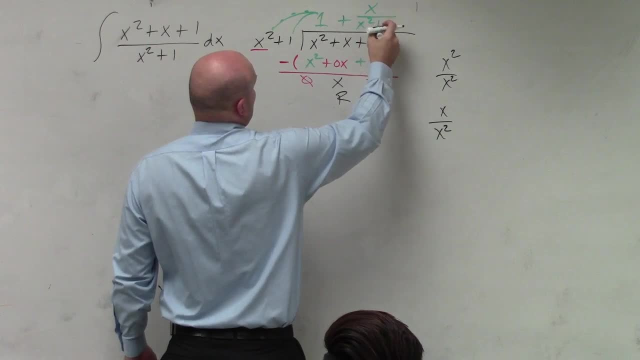 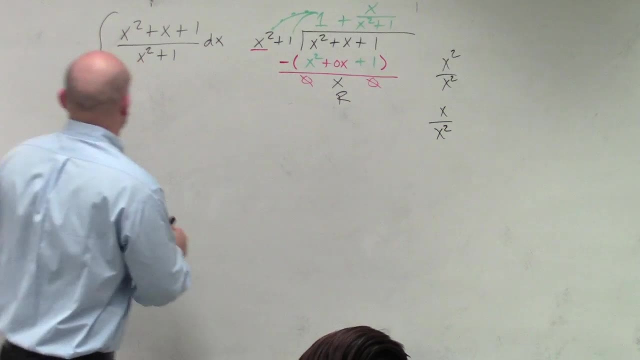 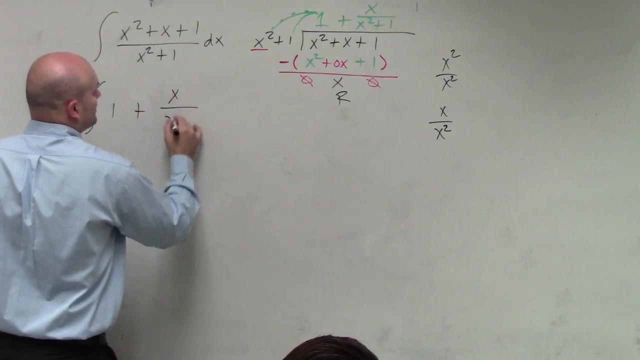 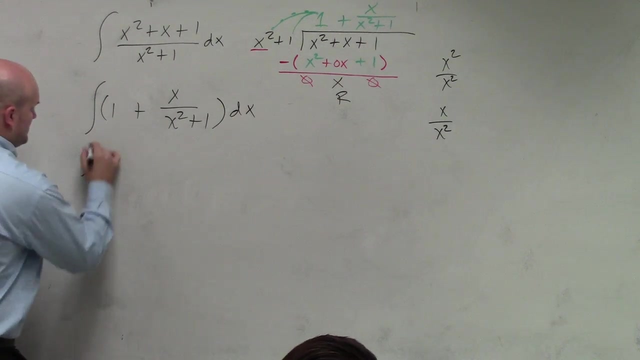 x over the divisor, x squared plus one, So you always take your remainder over your divisor, All right, So now let's go and write out, go back to our integral And let's write this as one plus x over x squared plus one, And I could rewrite this all as dx. So I could rewrite this as one dx. 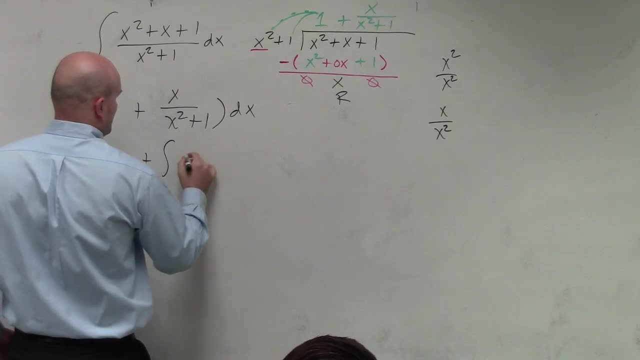 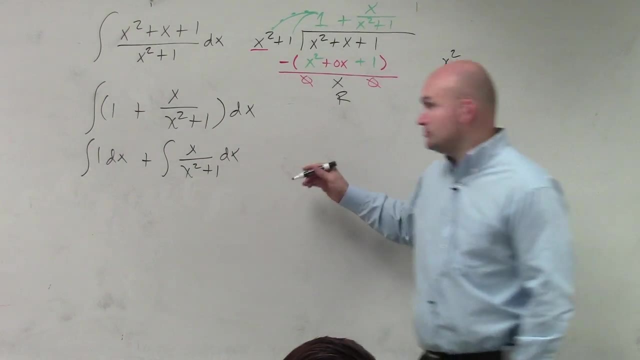 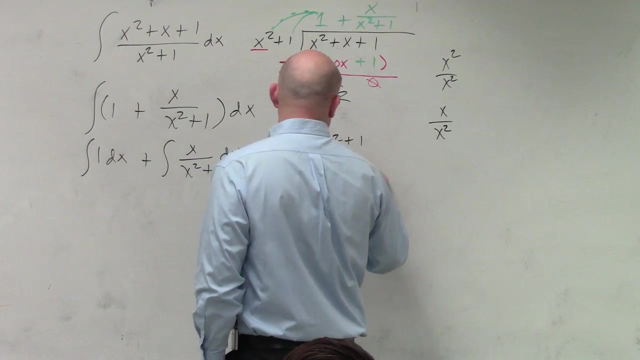 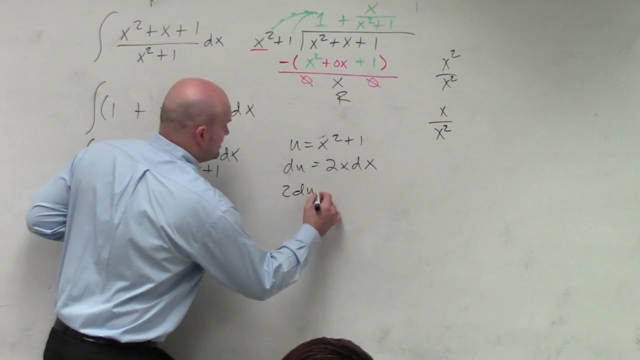 Plus over here I could see that ooh, x over x squared plus one dx, Whereas now I notice that for this I could use u substitution. So I could say: u equals x squared plus one. du is equal to 2x dx, where I don't have a 2, but I do have an x right. So I could say: 2 du is.